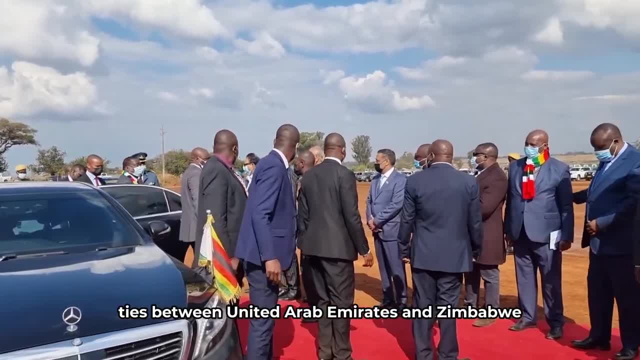 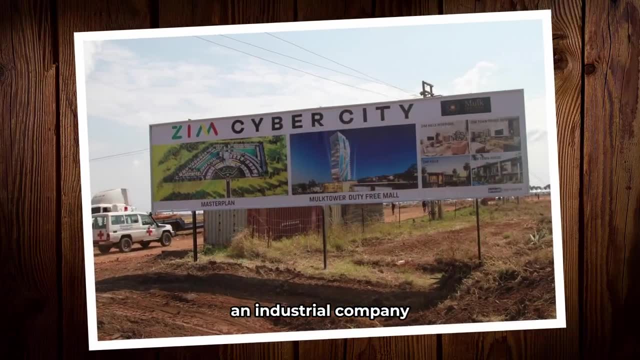 to the construction as a milestone project that will help bolster ties between Zimbabwe's construction and the United Arab Emirates during the groundbreaking event. Mork International, an industrial company located in the United Arab Emirates, is developing the project and investing about $500 million. 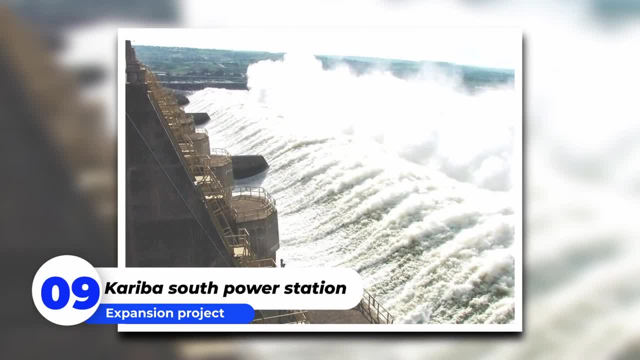 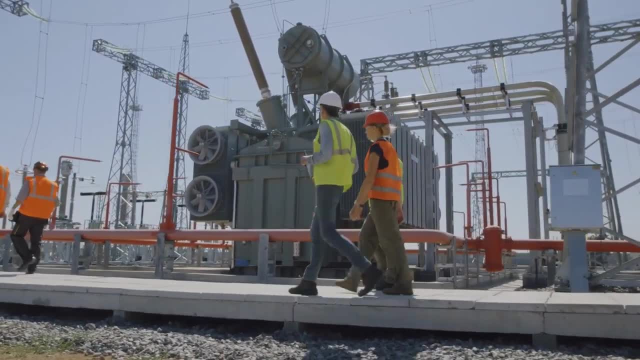 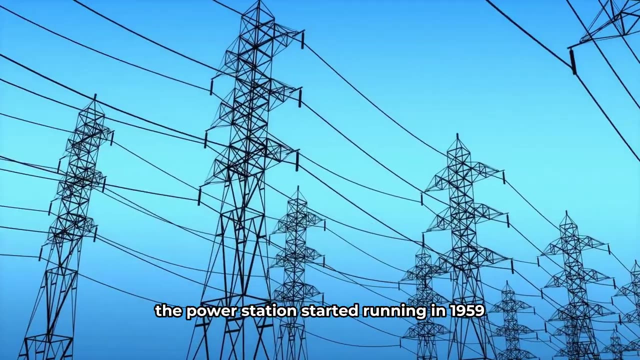 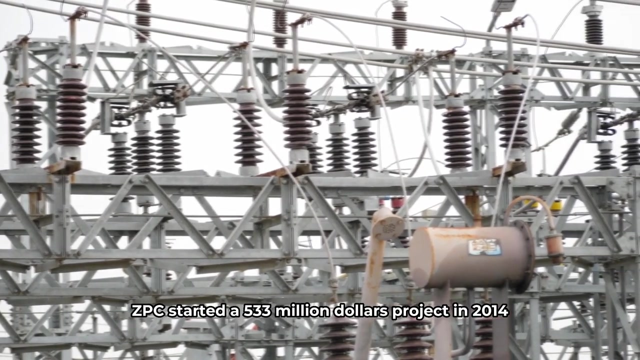 9. Kariba South Power Station Expansion Project. The largest source of residential electricity supply in Zimbabwe is the Kariba South Power Station, which is owned and run by the government of Zimbabwe-born Zimbabwe Power Company. The power station started running in 1959 and used 6 generator units to produce a round megawatts. ZPC started a $533 million project. 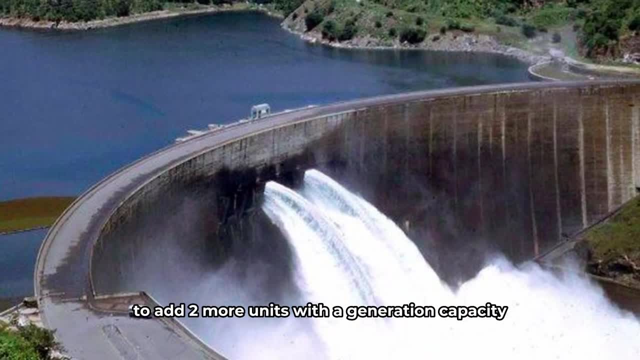 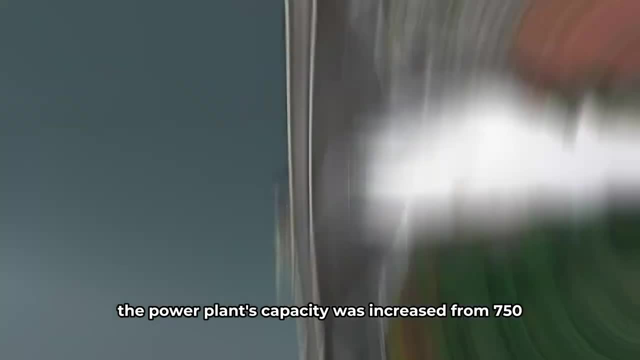 in 2014 to add two more units with a generation capacity of 150 megawatts each to the current facility. The power plant's capacity was increased from 750 megawatts to 1050 megawatts as a result of the problem, As after an sim immortalization operation, the power plant issued 250 megawatts for the Anwar Raum, a district andische towns site. The same grant. 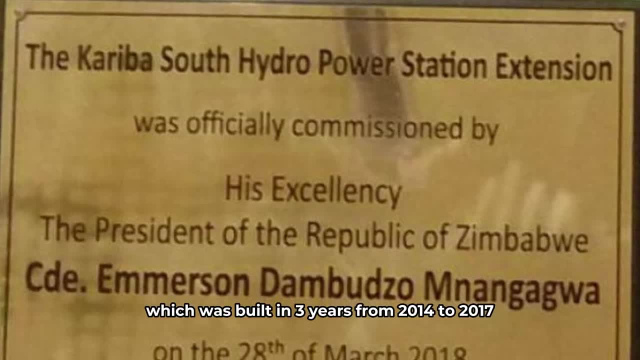 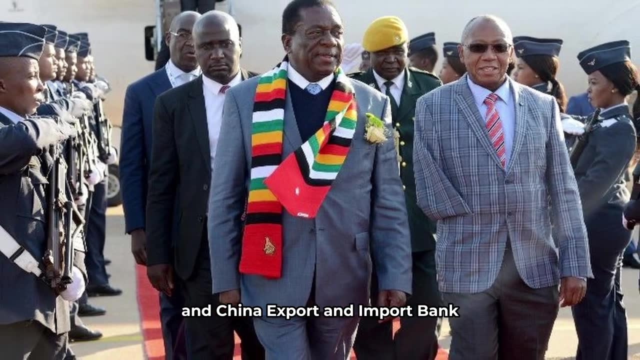 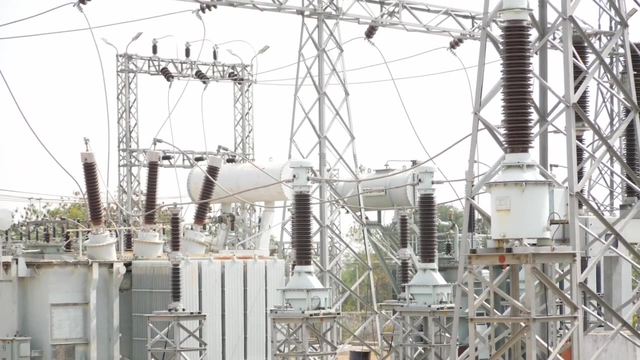 of the project, which was built in three years, from 2014 to 2017, by China's Sinhydro Corporation and co-financed by the Zimbabwean government and China Export and Import Bank. This helps the nation's supply of electricity. 8. Zimbabwe Roads Development Projects. 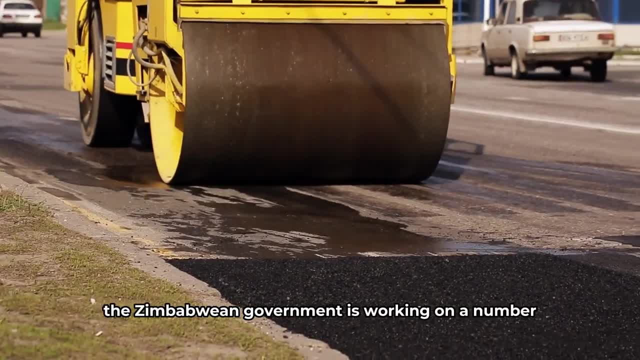 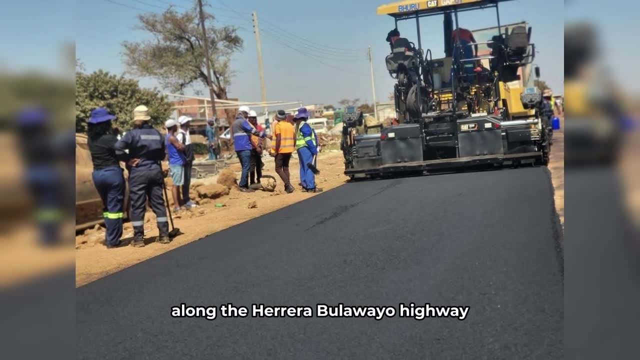 In an effort to update its road infrastructure, the Zimbabwean government is working on a number of significant road projects: Additional northern toll gates along the Herrera-Bulawayo Highway, as well as the dualization of the Herrera-Matari and Plumtree-Matari Highways. 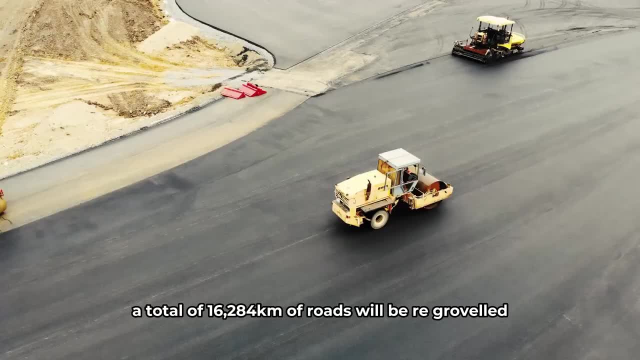 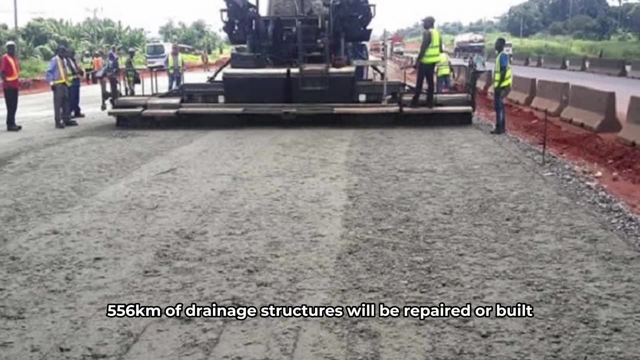 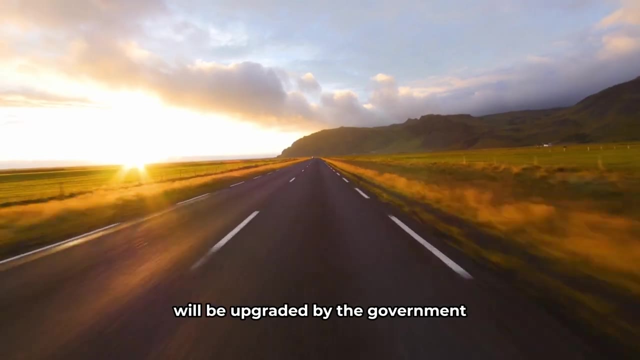 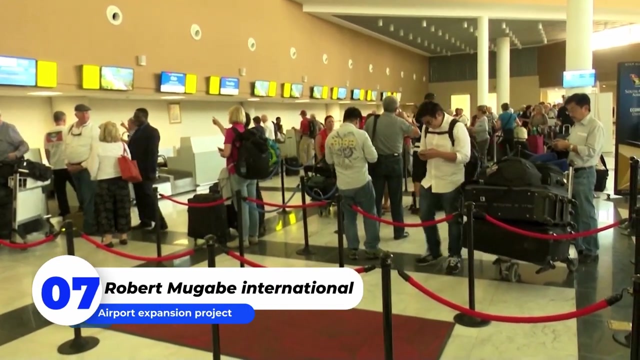 are also under construction. A total of 16,284 kilometers of roads will be re-graveled. 556 kilometers of drainage structures will be repaired or built. 22 bridges and other supporting infrastructure will be upgraded by the government. 7. Robert Mugabe International Airport Expansion Project. 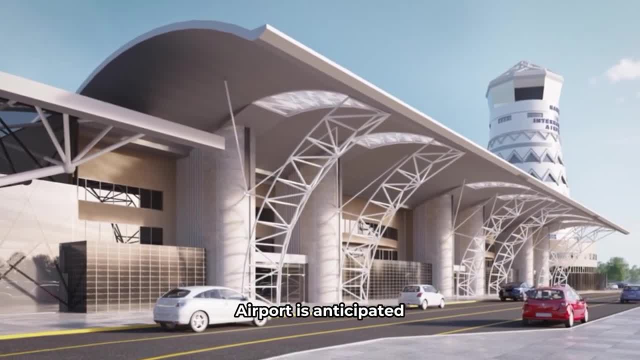 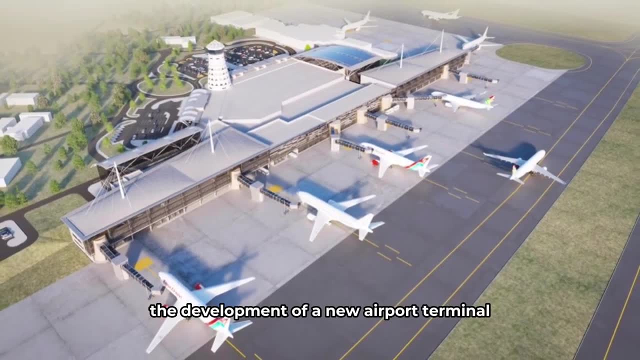 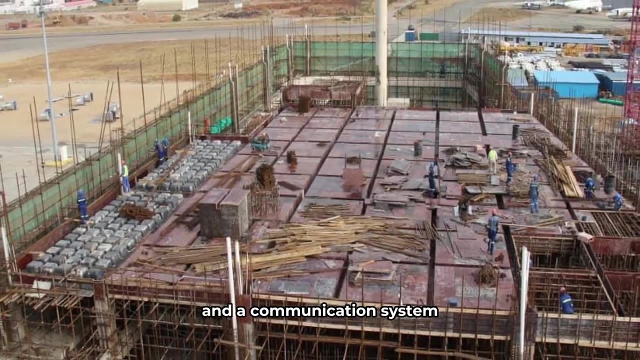 The development of Robert Mugabe International Airport is anticipated to greatly contribute to an increase in visitor numbers to Zimbabwe. The development of a new airport terminal, aprons for new bridges, a secondary radar system, an airstrip ground illumination and a communications system are all part of a $153 million project being carried out in Zimbabwe. China Export-Import Bank is providing funding for the project, which is being built by China Jansu International. The capacity of the airport to carry passengers is anticipated to expand from $2.5 million to $6 million annually, more than doubling. 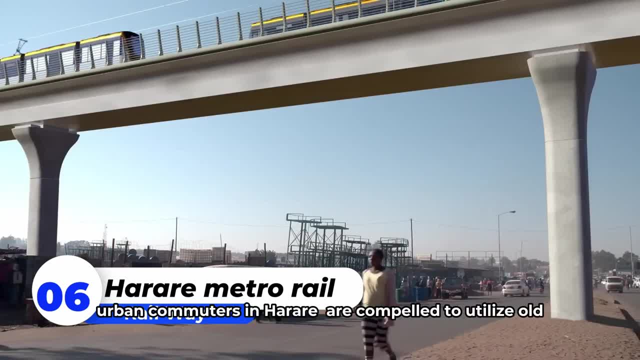 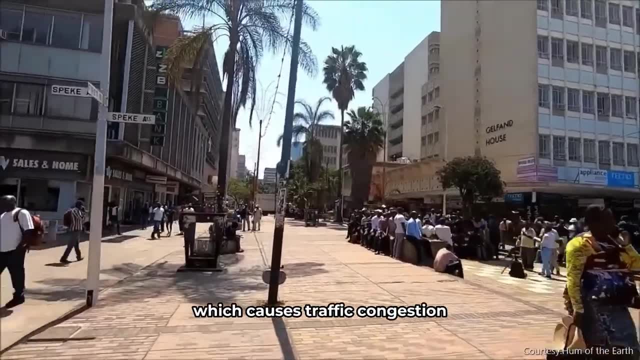 6. Herrera Metro Rail. Urban commuters in Herrera are compelled to utilize old, crammed cars because there are no other ways to transport passengers. The airport is a place where passengers can travel to other options, which causes traffic congestion, carbon emissions and traffic accidents. 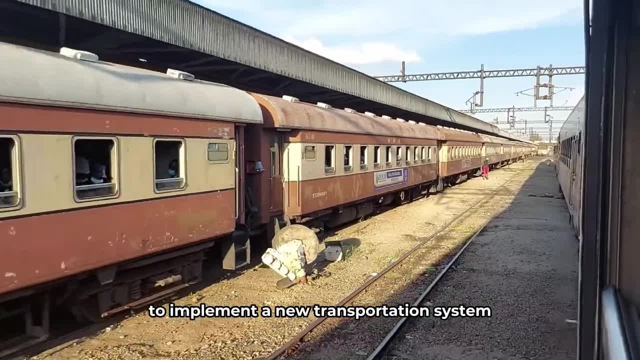 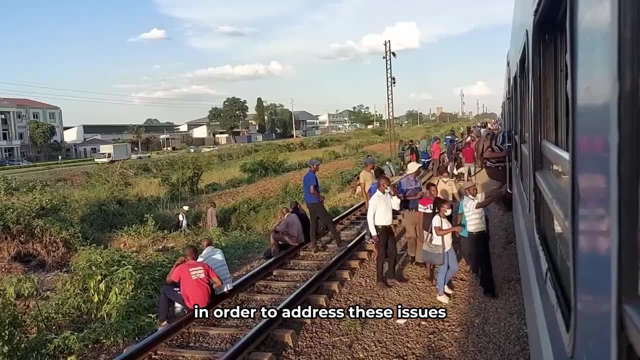 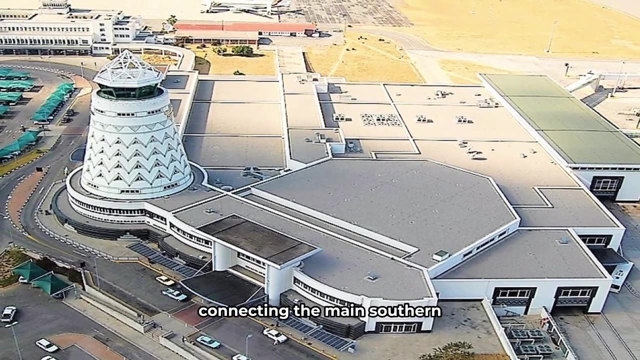 The Zimbabwean government intends to implement a new transportation system that will offer a dependable, safe and inexpensive public transportation option. in order to address these issues, The Herrera Metro was built in three phases. Phase 1 includes a 31 km railway line connecting the main southern high-density residential areas. Phase 2 includes building. 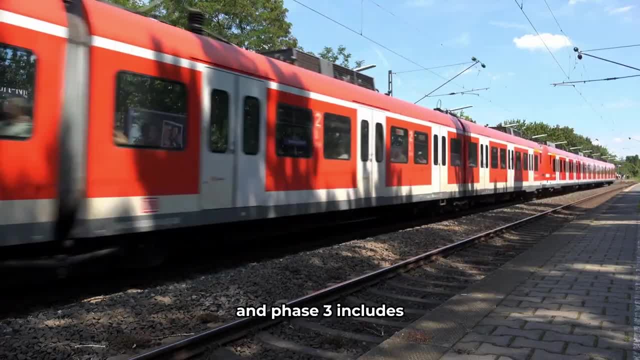 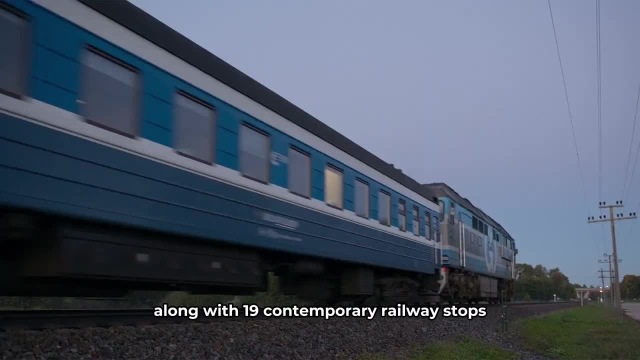 the line to Chichu, Makita and Mafumafu. Phase 3 includes the construction of a new railway line in Chichu, Makita and Mafumafu, And Phase 3 includes extending the line to the Robert Mungabe International Airport and the new parliament in Mount Hamden, Along with 19. 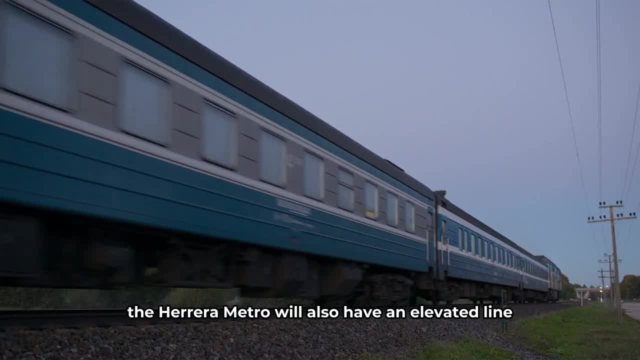 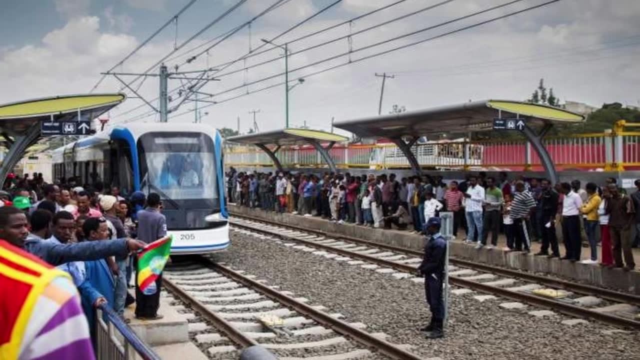 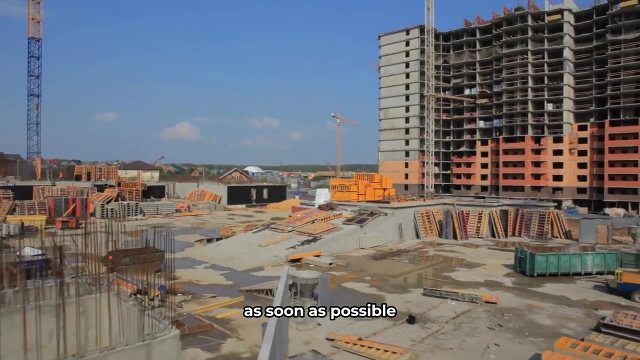 contemporary railway stops. the Herrera Metro will also have an elevated line that would assist it avoid obstructing city traffic. 5. Mount Hamden Smart City. Zimbabwe wants the newly constructed metropolis to open as soon as possible because it has been luring numerous investors. 5. Mount Hamden Smart City. 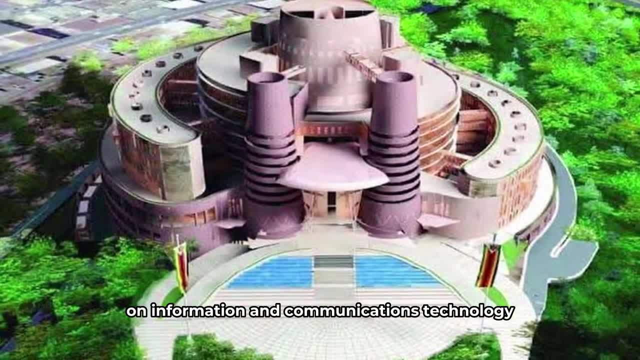 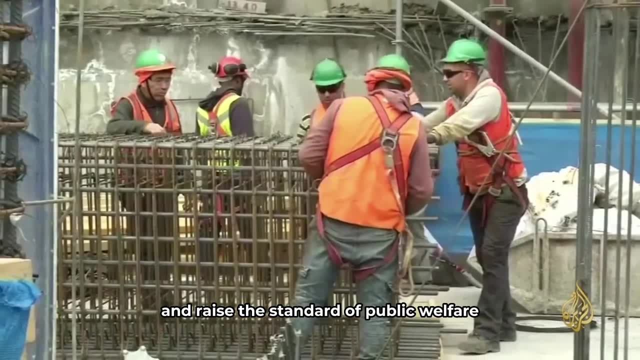 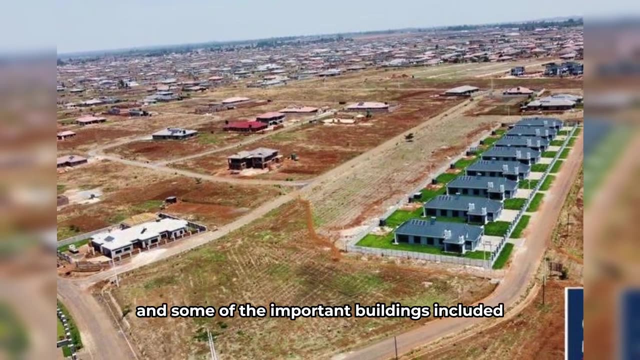 The newly constructed city places a strong emphasis on information and communications technology in order to increase operational efficiency and raise the standard of public welfare and government services. The master plan for the city was created by professionals from Herrera University, and some of the important buildings included in the design of the new city include: 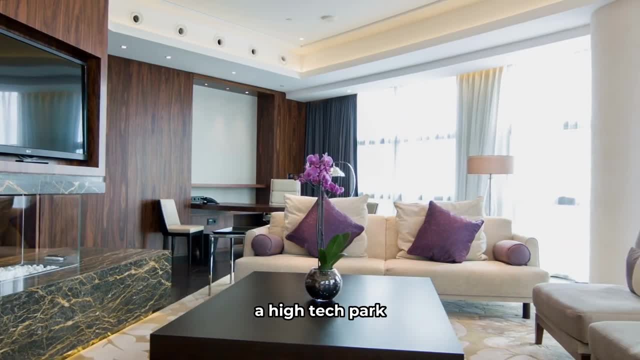 office parks, commercial entities, a high-tech park, information communication technology center, park, institutional facilities and a new city, 5. Mount Hamden Smart City, A city that provides services and services for the public and the community to the needs of all people. 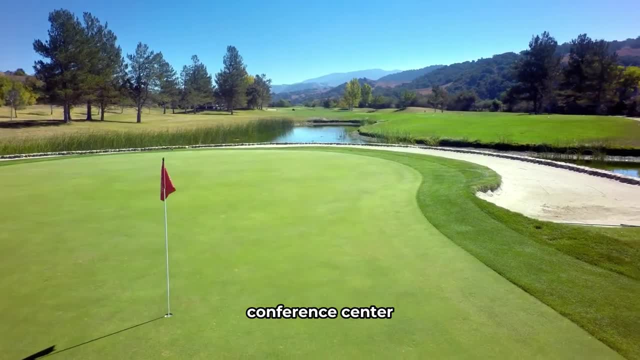 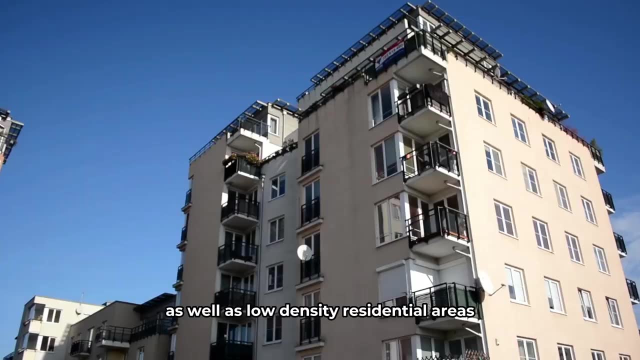 The city is a hub of cultural movements in the area of localization and social development: Agro processing buildings, resort hotels, conference center, golf course apartments, cluster houses and garden flats, as well as low-density residential areas, civic center and game sanctuaries. 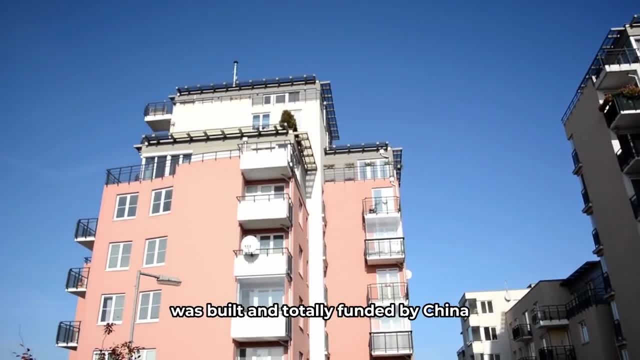 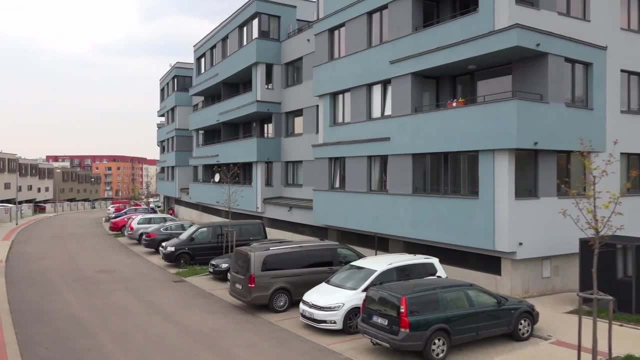 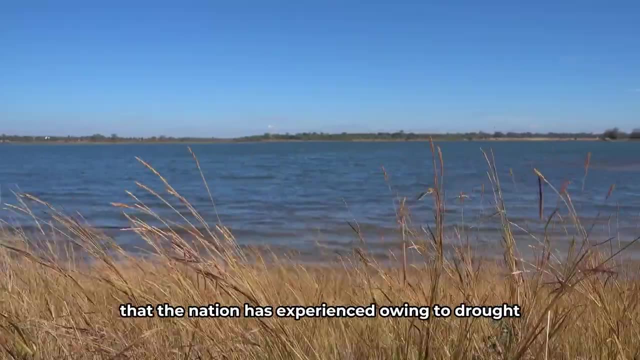 The new parliament building, which is central to the city, was built and totally funded by China as a present to the country of Zimbabwe. 4. Maybel Land- Zambrisi Water Project On order to address the recent water problem that the nation has experienced owing to drought. the Zimbabwean 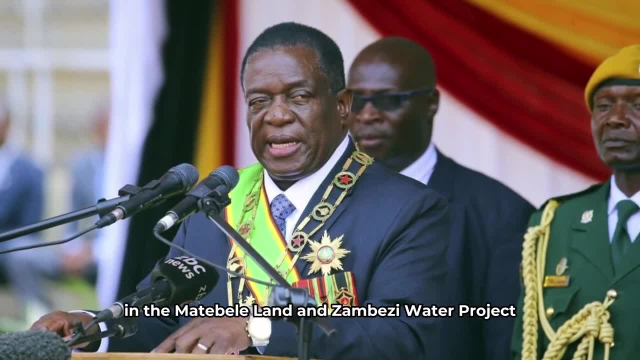 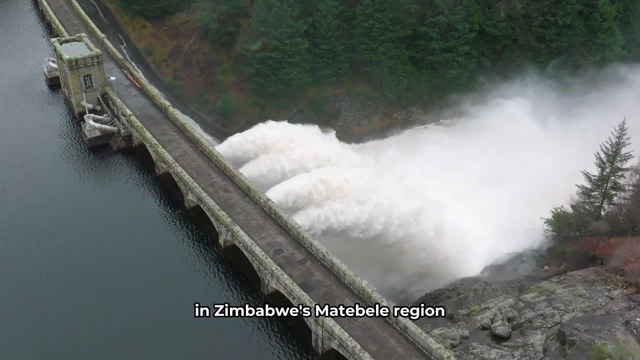 government is investing $600 million in the Maidbel land and Zambezi water project. The initiative entails a sizable water project in Zimbabwe's Maidbel region that intends to alleviate the ongoing water shortage plaguing Bulaweo, the country's second-largest city. 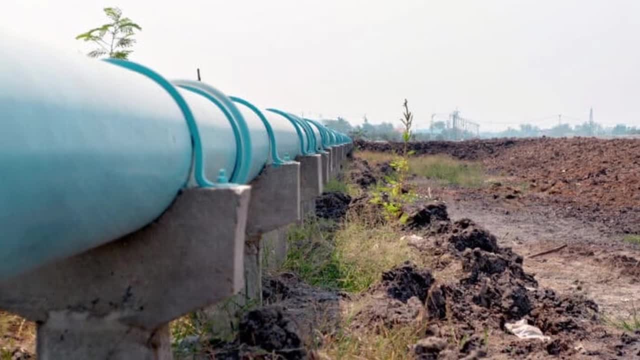 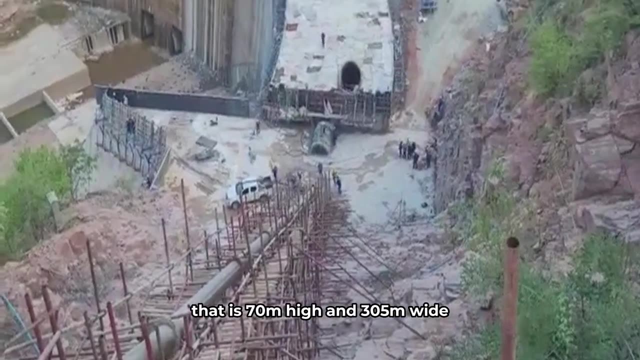 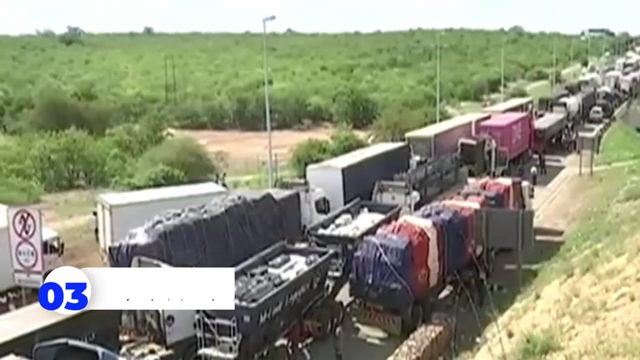 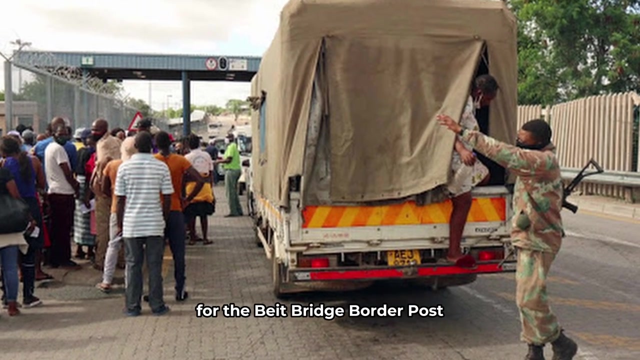 by supplying water from the magnificent Zambezi River. The dam is a 634 million cubic meter roller compacted concrete gravity structure that is 70 meters high and 305 meters wide. 3. Bait Bridge Border Post. The 930-kilometer upgrading project for the Bait Bridge Border Post includes a border post. 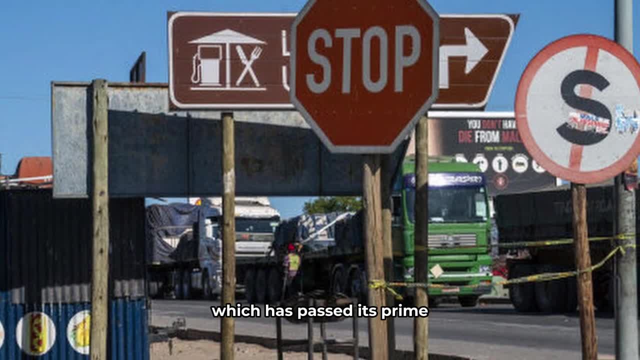 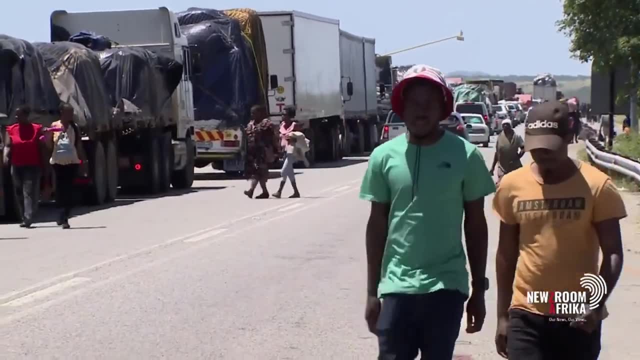 at Bait Bridge. The quality of the road, which has passed its prime, is anticipated to improve with the completion of the highway. There are two phases to the project. In fact, the Bait Bridge Border Post is a project that will be completed in the next. 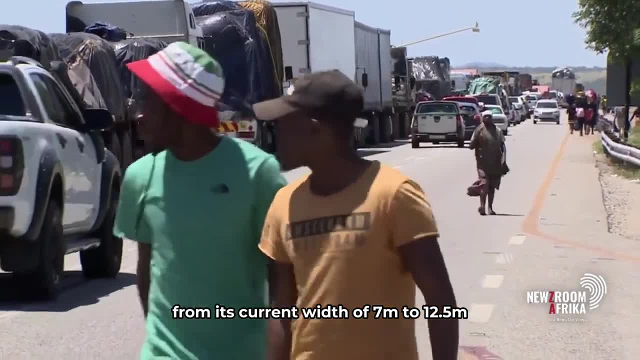 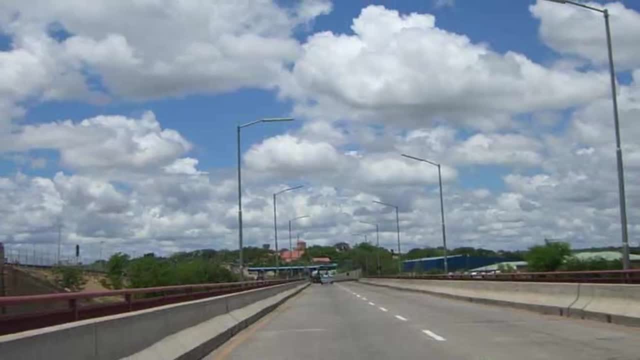 phase. Phase 1, the roadway will be widened from its current width of 7 meters to 12.5 meters, in accordance with Southern African transport and communications requirements. Phase 2 of the project will see the construction of a fire station, residential buildings, a sewage dam. 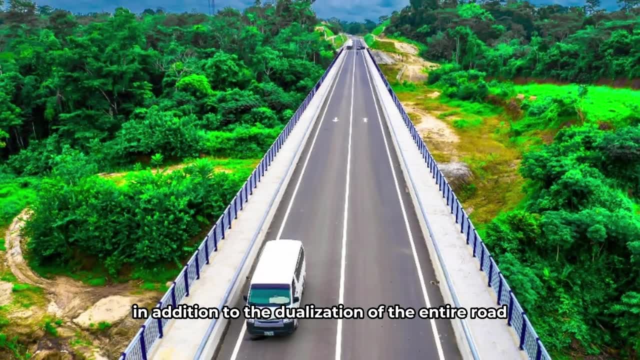 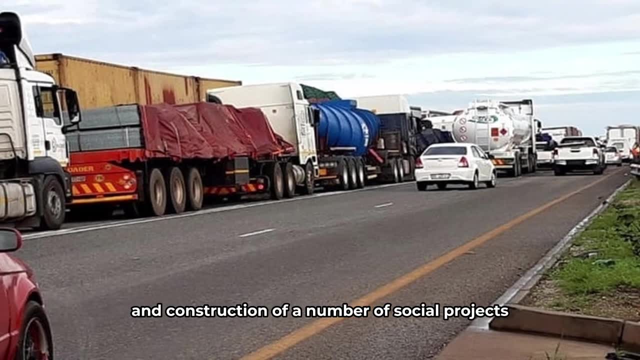 and a new water reservoir, in addition to the dualization of the entire road, renovation of the entire border post, ICT infrastructure and construction of a number of social projects. The construction is being done by the Bait Bridge Border Post, which is a project that is being 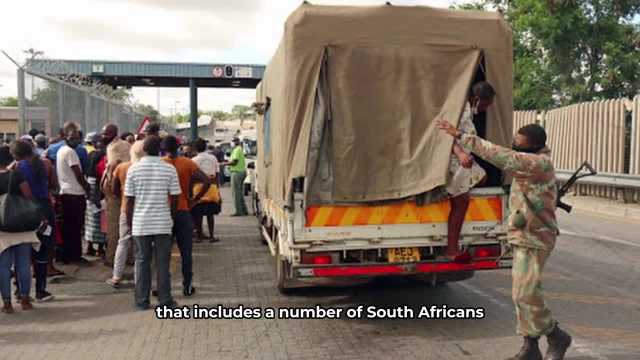 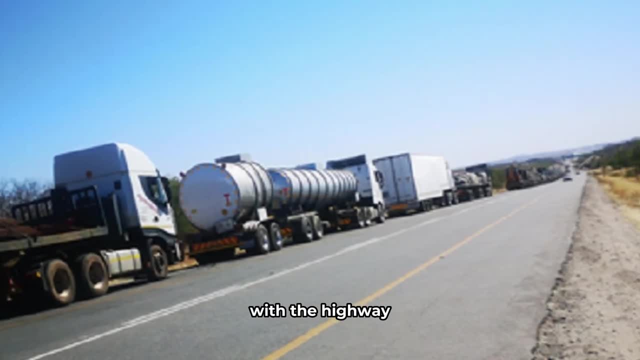 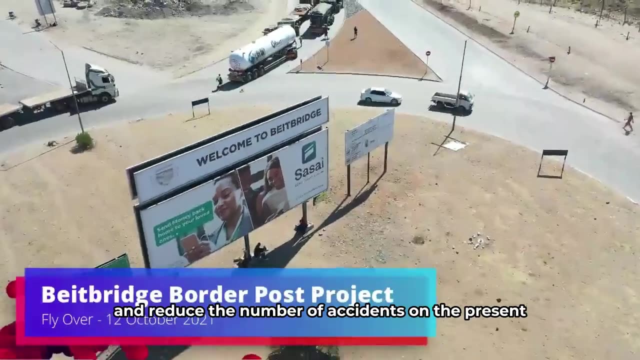 done by a collaboration that includes a number of South Africans, Zimbabweans and business people from other countries, professionals and financial organizations. With the highway, Zimbabwe will be able to make use of its strategic location to serve as a regional logistics hub and reduce 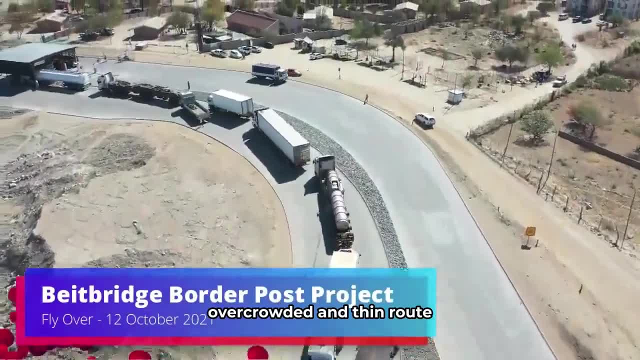 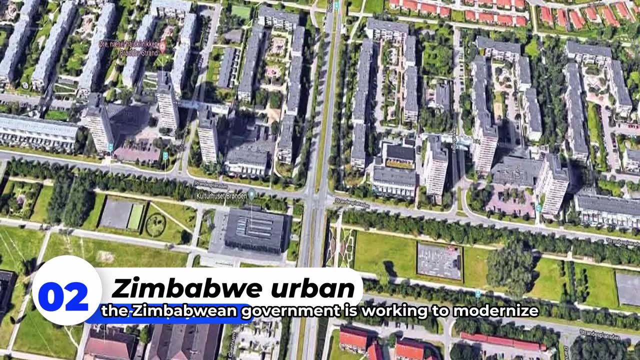 the number of accidents on the present overcrowded and thin route. 2. Zimbabwe Urban Renewal Projects. The Zimbabwean government is working to model a new road for the Zimbabwean government. The Zimbabwean government is working to model a new road for the Zimbabwean government. 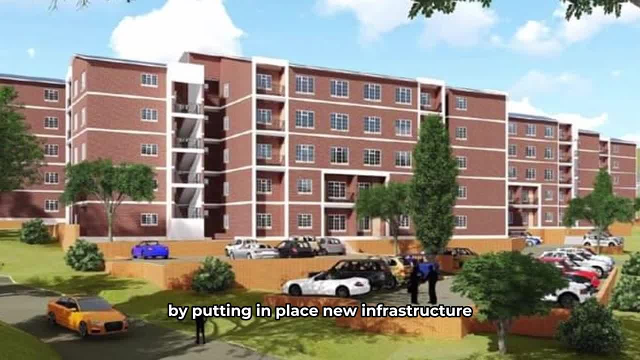 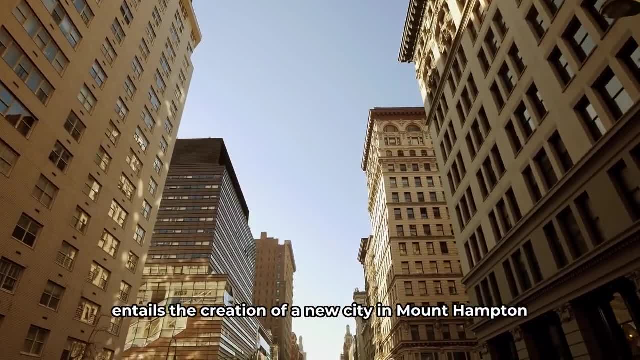 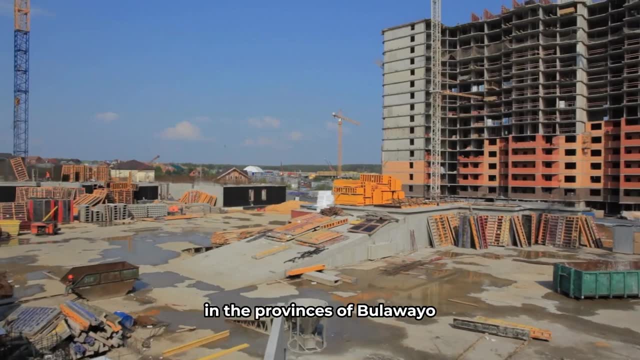 The project entails the creation of a new city in Mount Hamden and a satellite town on the outskirts of Victoria Falls, as well as the development of housing infrastructure in the provinces of Bulaweo, Harare, Masfingo and Matari.